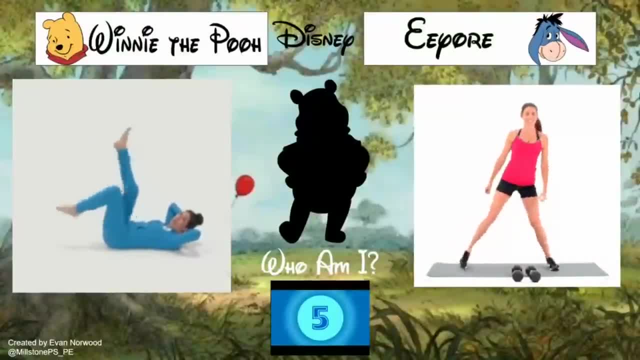 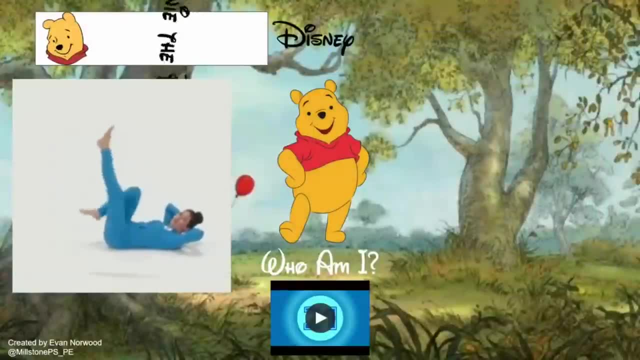 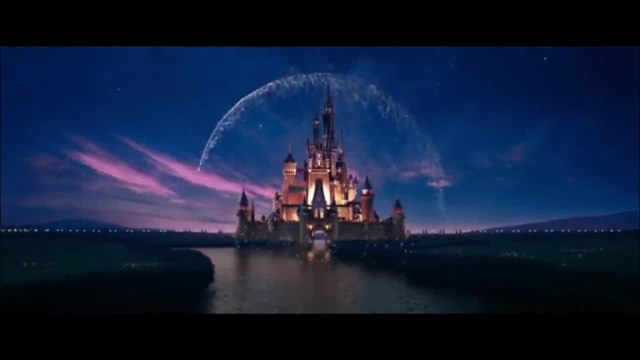 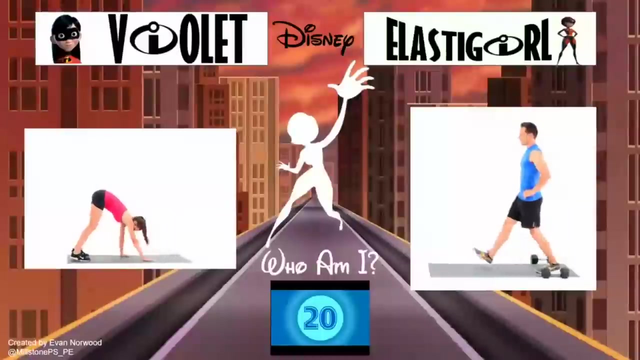 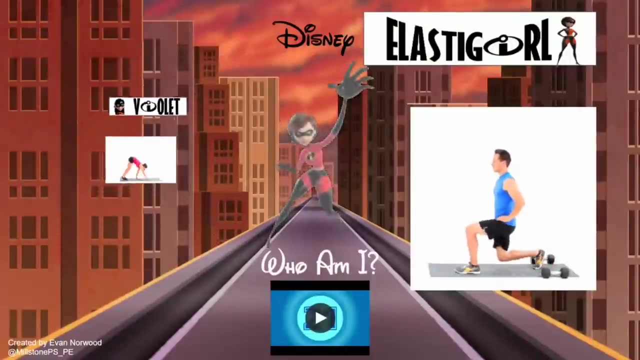 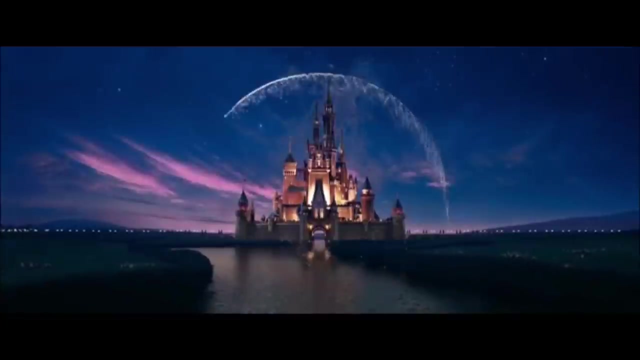 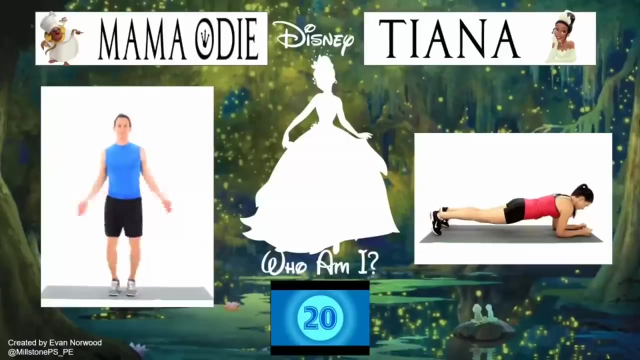 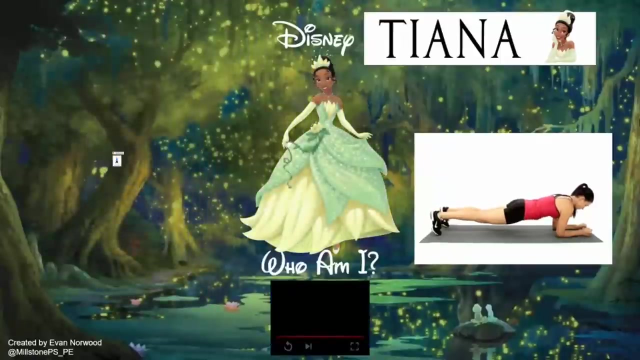 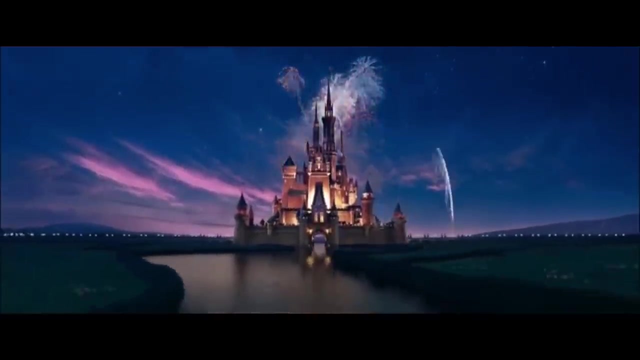 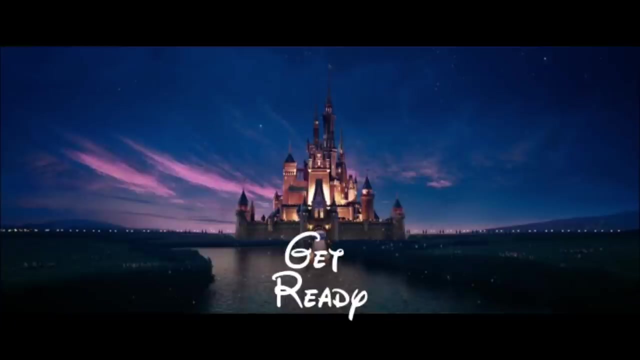 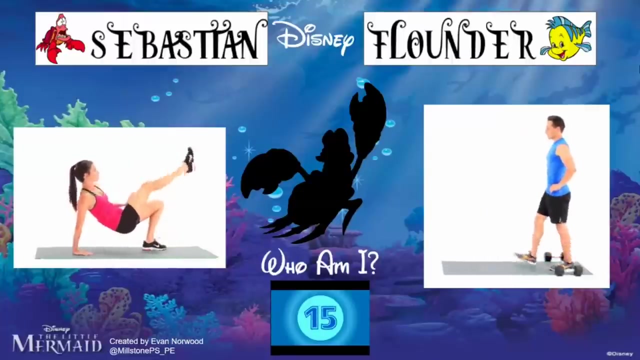 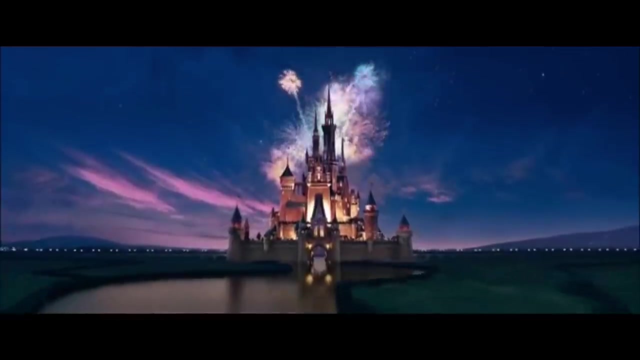 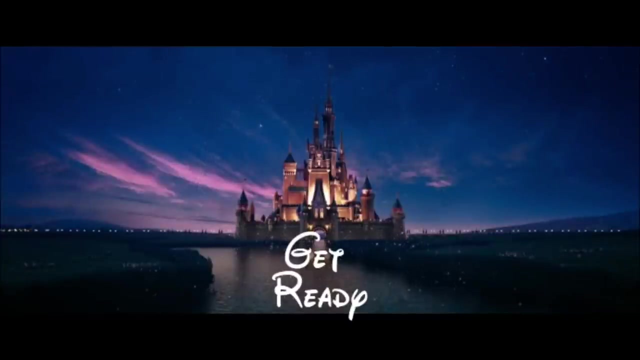 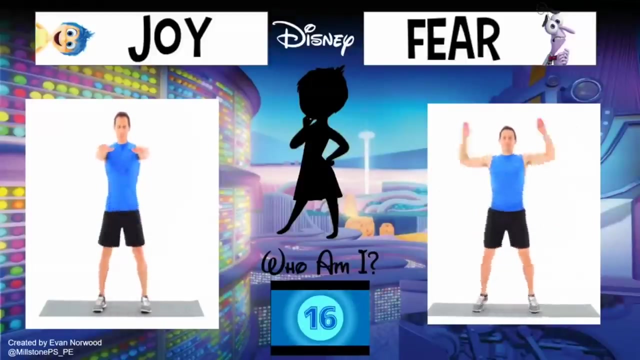 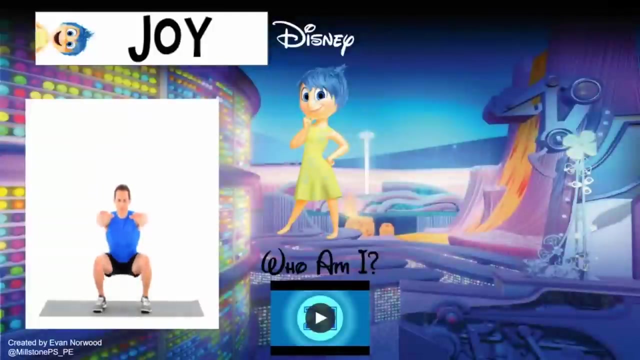 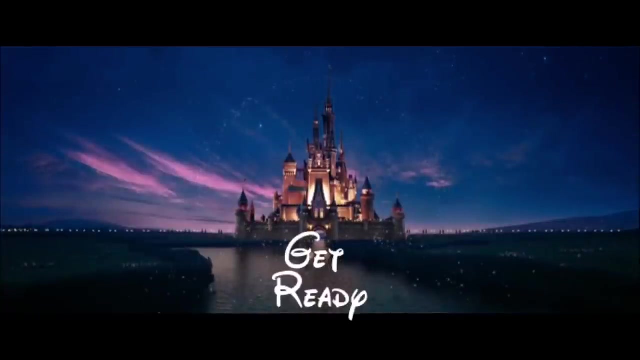 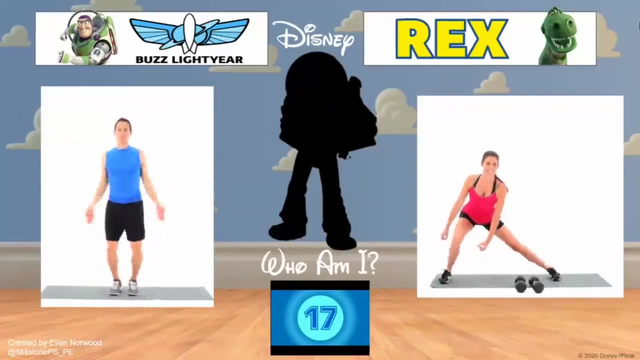 Thank you for watching. Thank you for watching. I've climbed a mountain, I've crossed a river And I'm almost there. I'm almost there. I'm almost there. Thank you, Thank you, Thank you. You've got a friend in me.